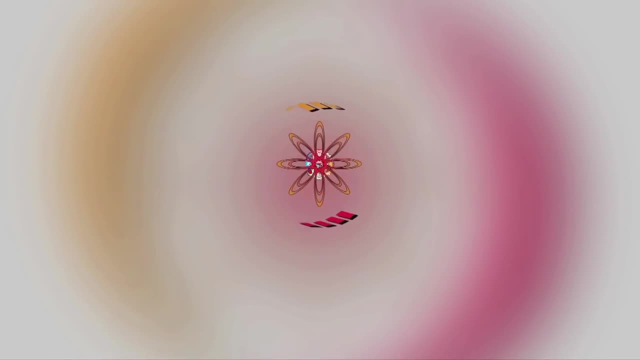 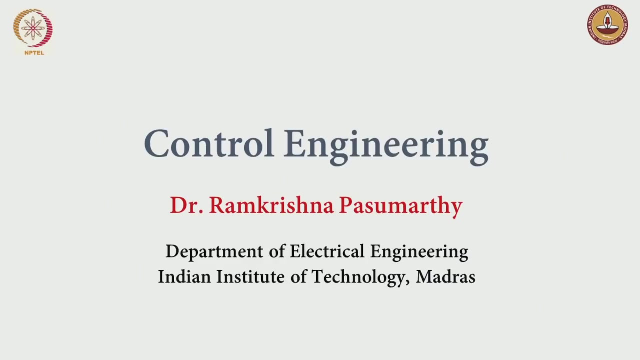 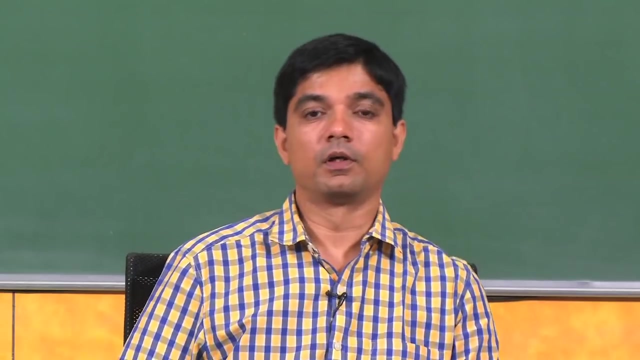 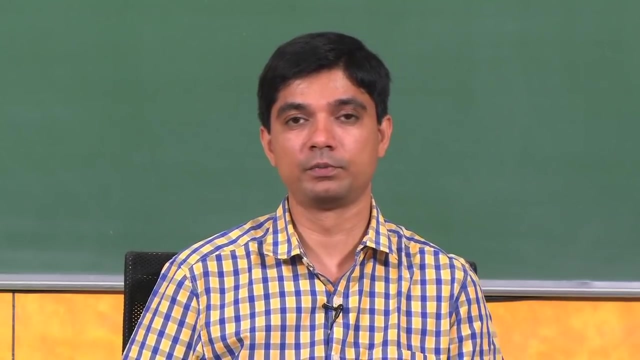 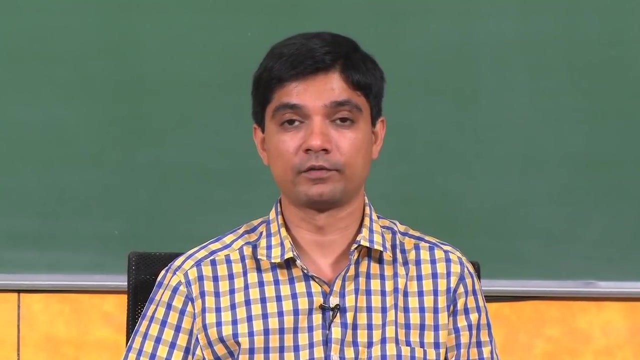 In the previous class we concluded with the concept of relative stability that if I want my poles to be not in the left half plane but left of minus 1, can I do that, or does my Routh Hurwitz criterion give me an answer to that? The answer was yes, you know I could. 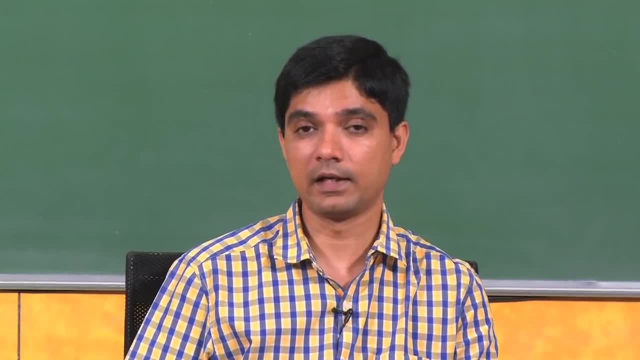 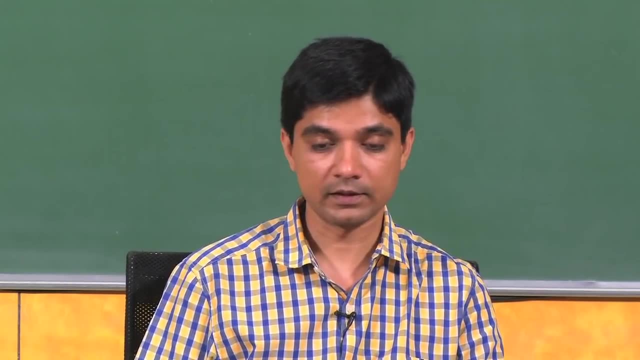 find out if the roots are to the left of minus 1, sati, to the right or on the axis itself. but that may not necessarily be enough when I am handling design problems right. So what we will do today is to learn a technique called the root locus, which will tell me little. 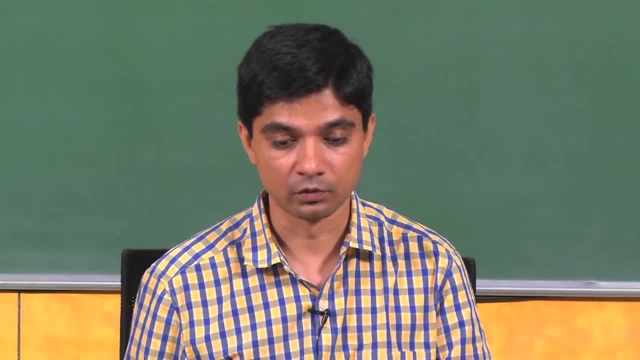 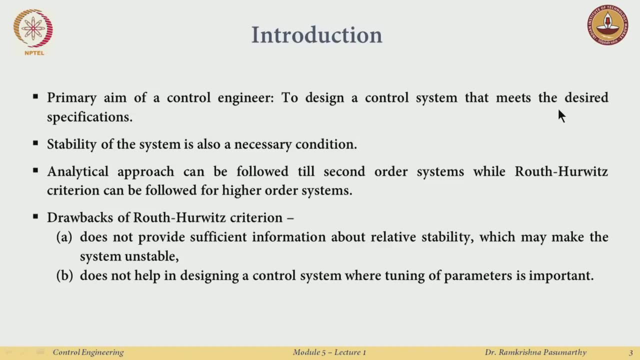 more about relative stability, right. So what is this root locus all about? So when I design a system, so I want the system to be such that it meets the desired specifications. And if we go to our earlier lectures, the specifications were usually either in the 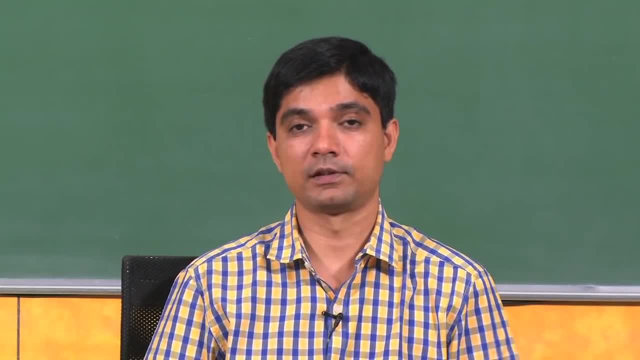 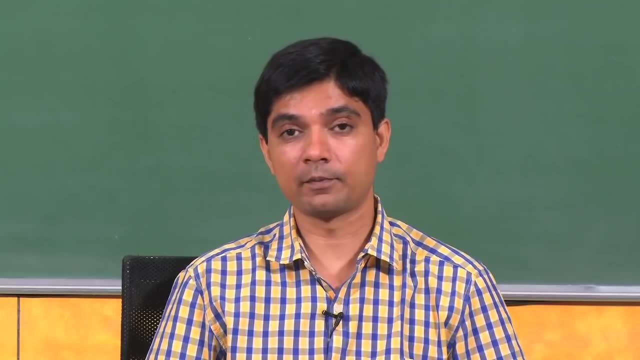 transient response or in the steady state response. So in the transient response I wanted to speed up the response, but then I had a constraint of the overshoot, So I wanted to speed up, So in such a way that I do not overshoot too much, and I also wanted the system to have 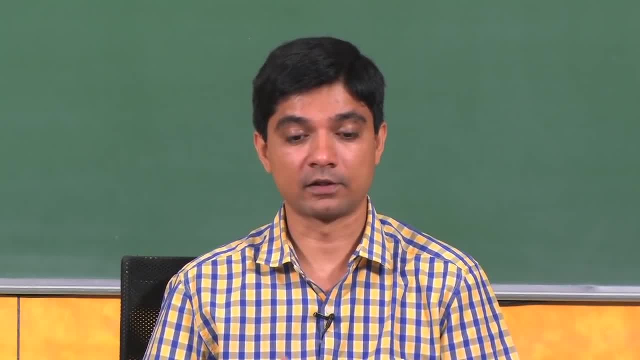 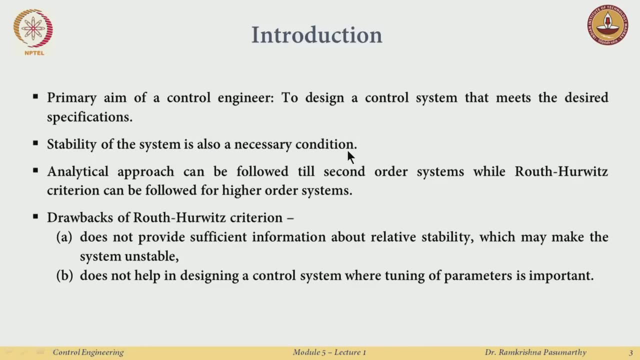 well, very small or no steady state error at all. But before I do this, I always wanted that the system should first be stable. If it is stable, then I can look at performance right. So until now, what we did? We just followed some analytical approach while we 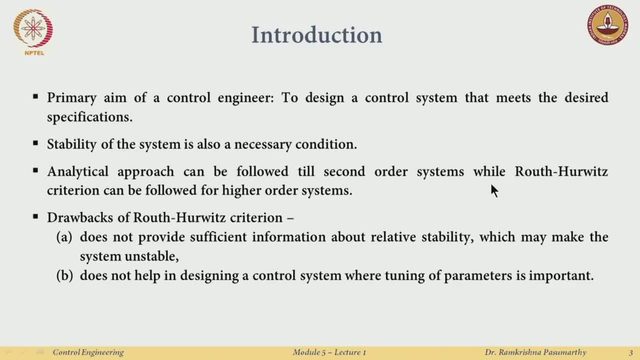 do while we were doing the Routh Hurwitz criterion. So it does not provide, even though it gives me some information of relative stability. 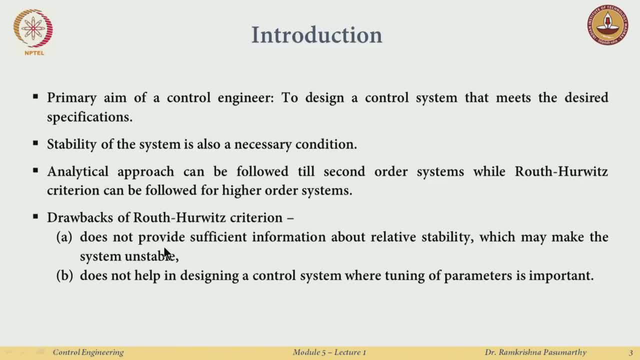 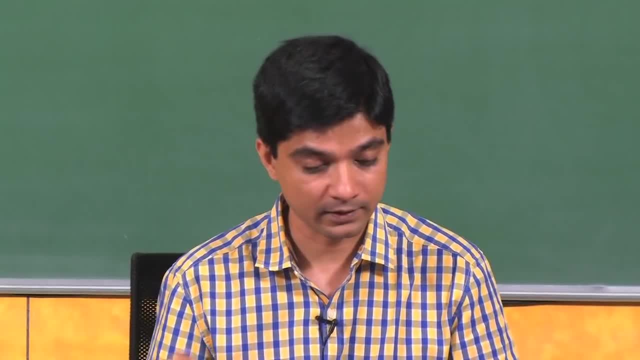 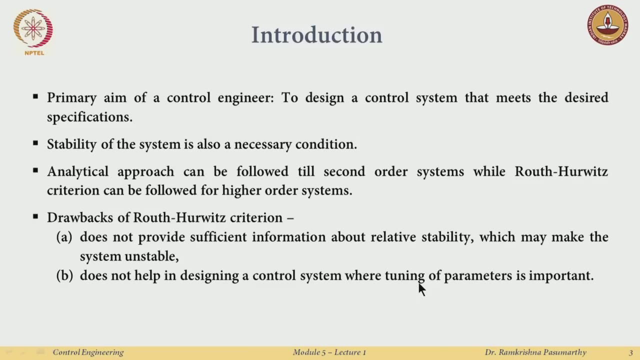 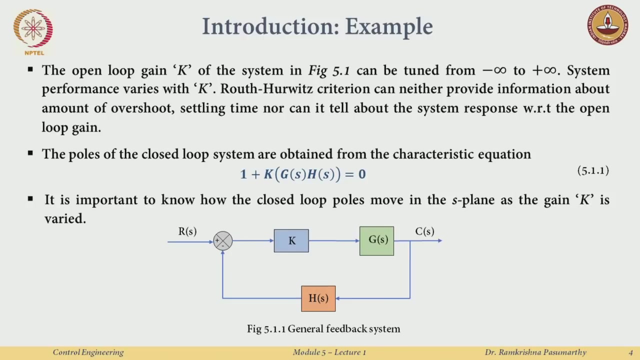 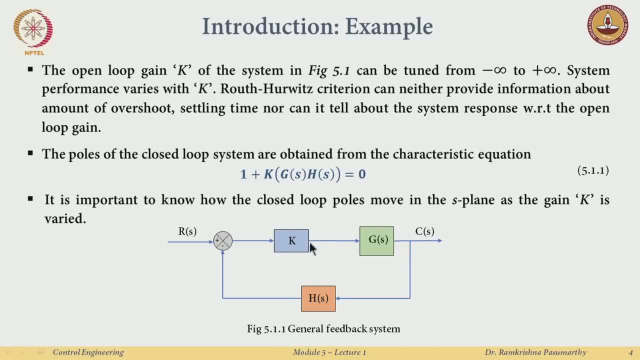 Right, and I just ask a question: what happens if I change this gain? It could be from all values possible, values from minus infinity to zero, and 2 plus infinity. What happens to the system? Well, the Routhorois does not really give me an exact answer to this question, neither. 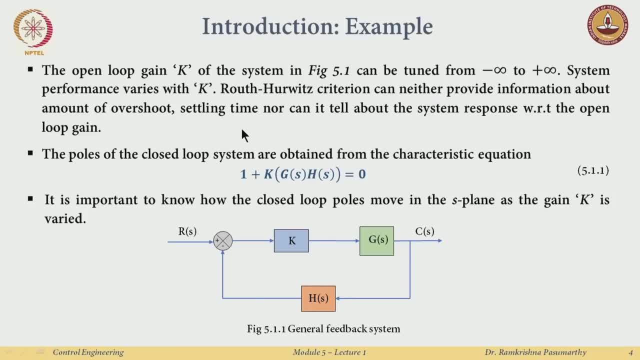 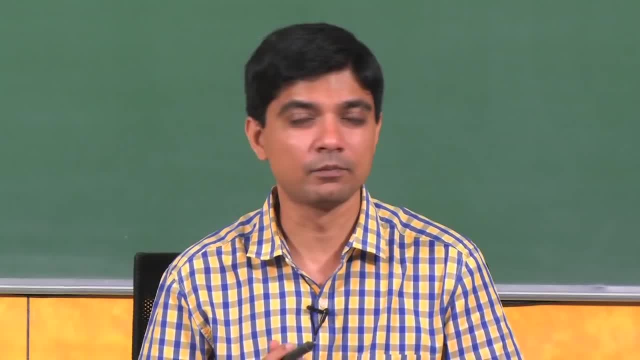 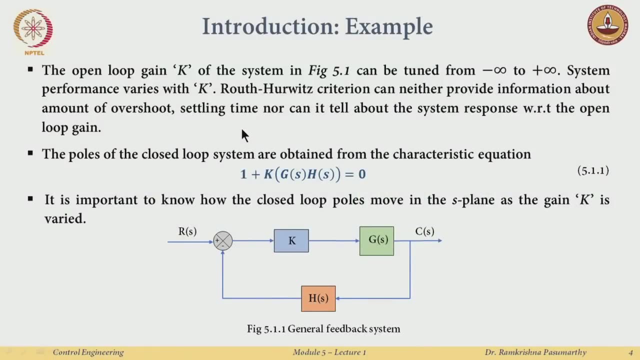 does it tell me any information about the settling time or the rise time, overshoot or even the steady state error, right? So for those things I need something little more sophisticated or little more in detail, right, ok, So let us see. are there any techniques? 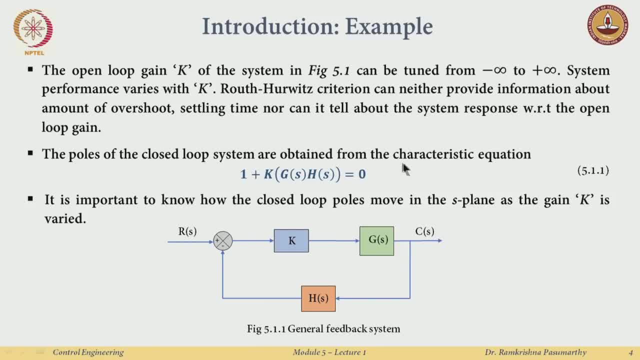 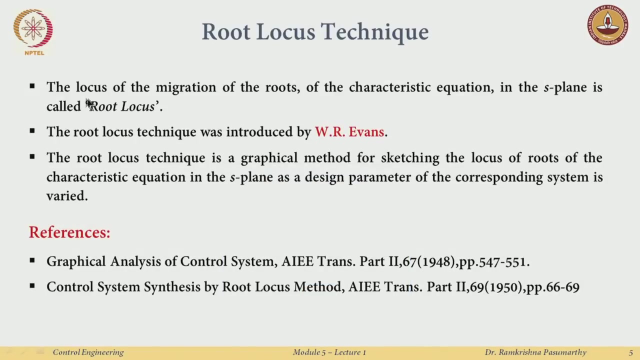 like that, right. So as again. so what we will be interested is in the characteristic equation, the solutions of which will give me the location of poles of the closed loop system. So we would like to know how the poles of the closed loop system vary by changing the gain k. ok, So this thing, this the locus of 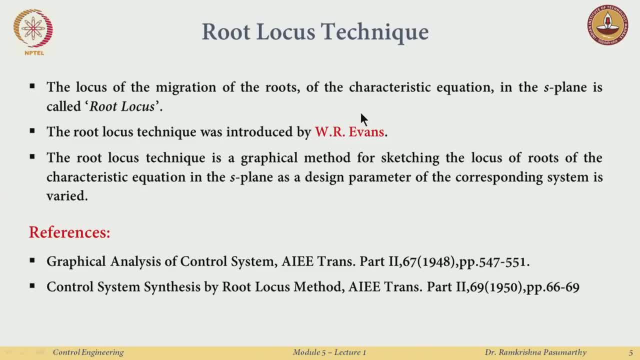 the migration of the roots of the characteristic equation as the gain k varies, is called the root locus techniques, introduced by W R Evans in his paper in 1948.. So what is this guy? This root locus is a technique. it is a graphical. 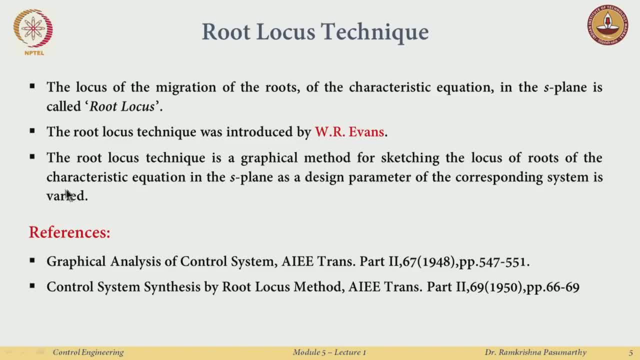 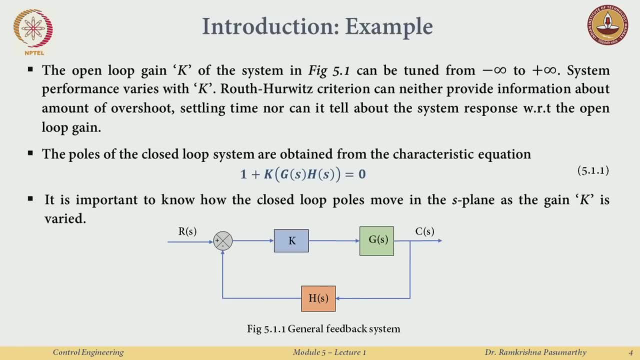 technique. So what is this guy? This root locus is a technique. it is a graphical technique For sketching the locus of the roots of the characteristic equation as a certain design parameter. here it is this: gain k. it could be something else also. we will see how we. 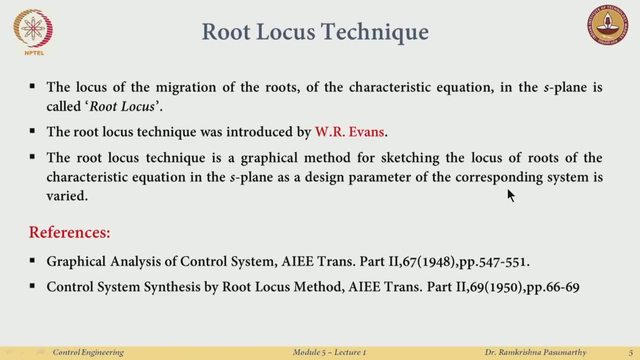 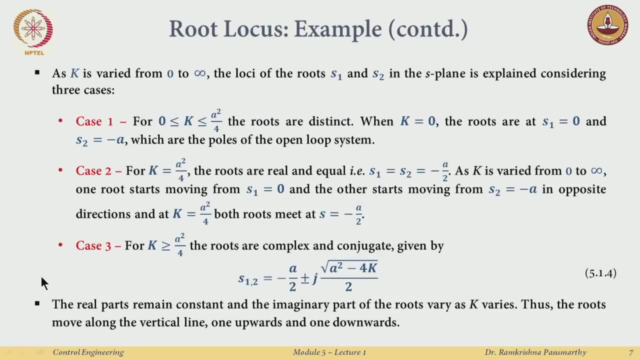 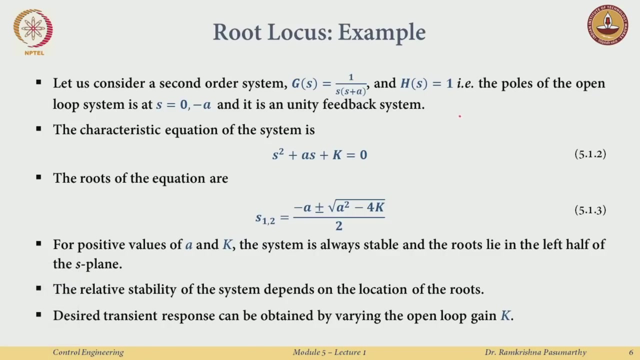 deal with those when this design parameter is varied, and these are the first two papers where this root locus was first introduced. ok, So let us not get into that at the moment. let us start with something very small, right? So I start with a second order system. if I were just to draw it, I have in my forward 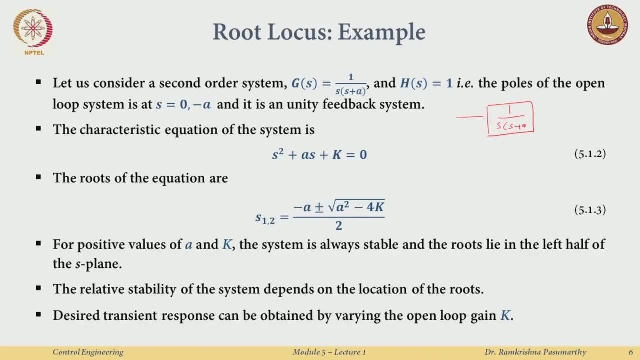 transfer function 1 over S, S plus a, I have H of S is 1, a plus a, minus. here again, all these usual things of R and C as 1, right. So the characteristic equation- here I am equation of the system, 1 plus g, h equal to 0, gives me something like this: ok, Now the 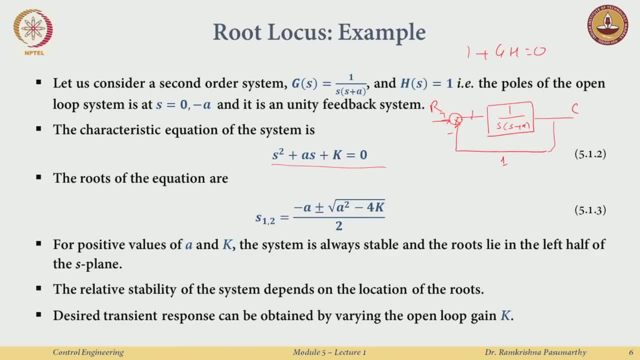 roots ok. So I think I should also put a put a gain k here. another block: ok. So this will give me the characteristic equation in this way. So the roots of this equation. second order equation: I have 2 roots minus a plus minus square root, a square minus 4 k over. 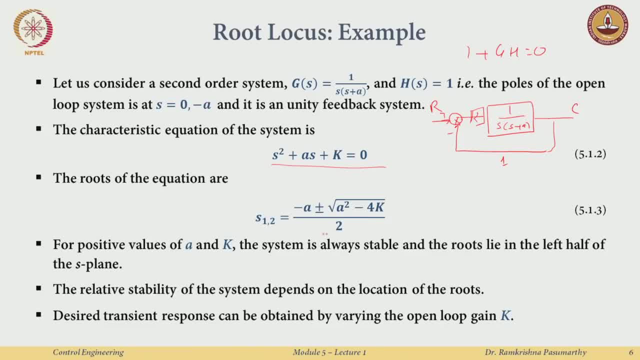 2. ok, So let us analyze what this, how these roots change and what are the two parameters here: a changes and k changes. ok, So for positive values of a right, when a is greater than 0, minus a is always less than 0.. Additionally, if k is also greater than 0, system is always 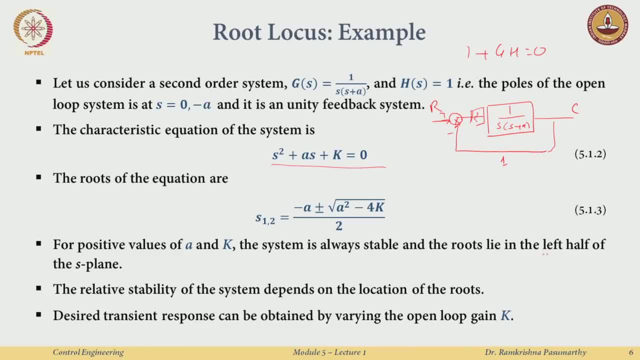 stable right. and because this guy right? because- and the root, always roots of the system always lie in the left half The relative stability now depends on the location of the roots right. So then I could see that by varying k, which is corresponds to my omega n in the second order analysis. 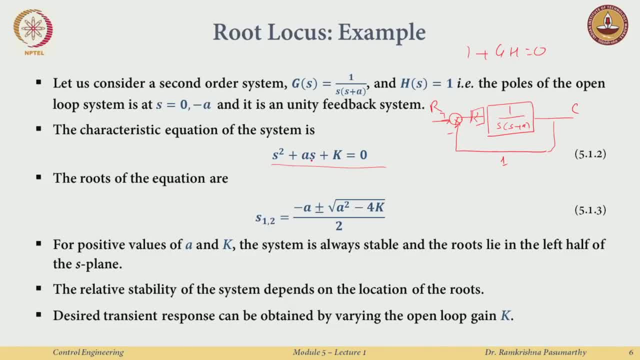 this guy corresponds to 2 zeta omega n. you know, dealing with the damping coefficient also right. So the desired transient response can be obtained by just changing this if the a is fixed. right, So, given a transfer function, a could be fixed. 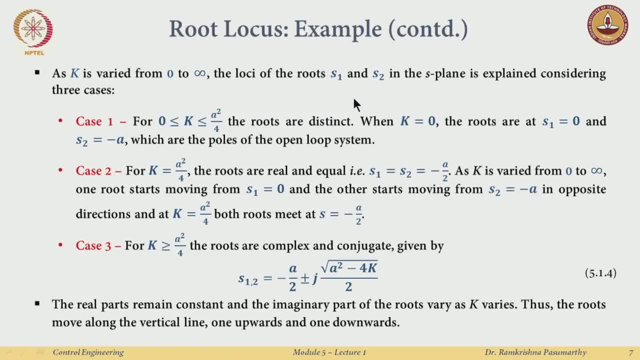 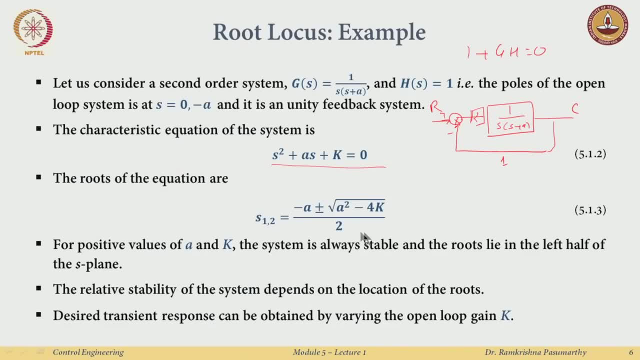 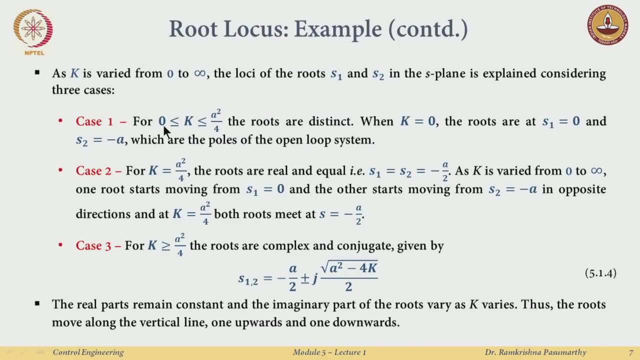 So what happens? So, given a, there could be few cases, because the roots of the characteristic equation depend on what is the sign of this guy. ok, So for case 1, when k is between 0 and a square by 4, the roots are distinct. 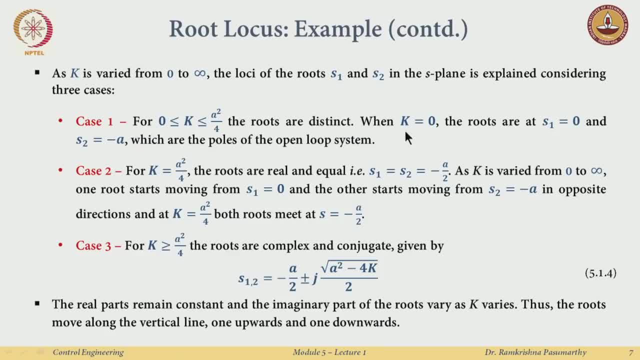 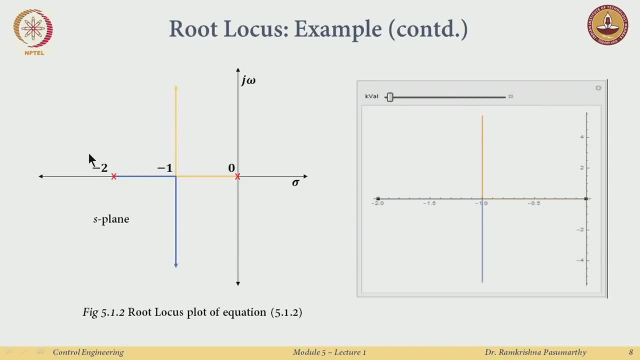 are distinct, right? I can just see very easily When k equal to 0, the roots are at s 1 equal to 0 and s 2 equal to a. ok, So let us plot that for right. So this may plot it here. 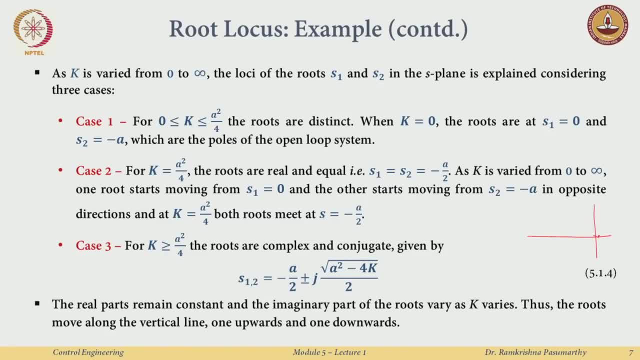 right. So I start with k equal to 0,. I am here, that is a 0, and I am here, this is minus k in the s plane sigma and j omega right For k between 0 and a square by 4 right. So. 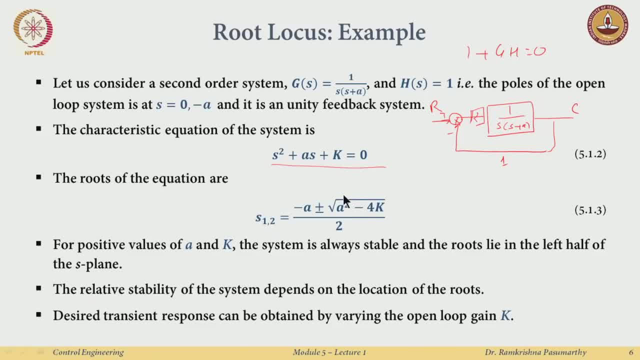 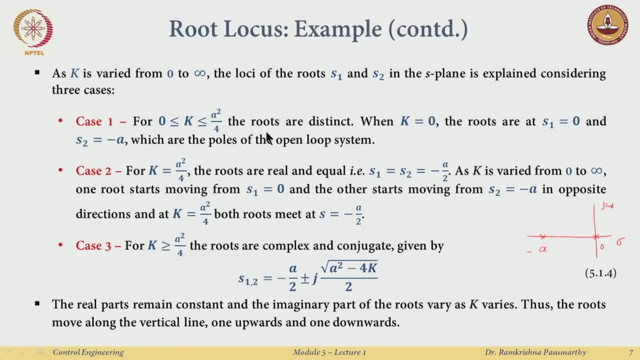 this guy would be real in that case, right, So the roots would be distinct. ok, So there will be somewhere. I know that there will be distinct. they will just be real. this and somewhere on this in this axis could be here and wherever, but I know that I have a stability. 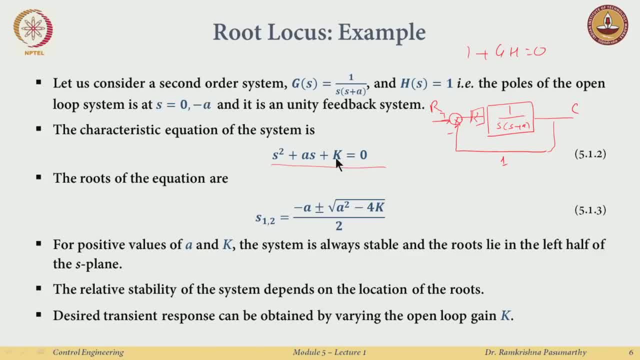 So stability is always maintained because a and k are positive. you do not even need to look at the route table right here. maybe you can just trivially see that the route condition is satisfied. And therefore, when we were doing the second order system analysis. 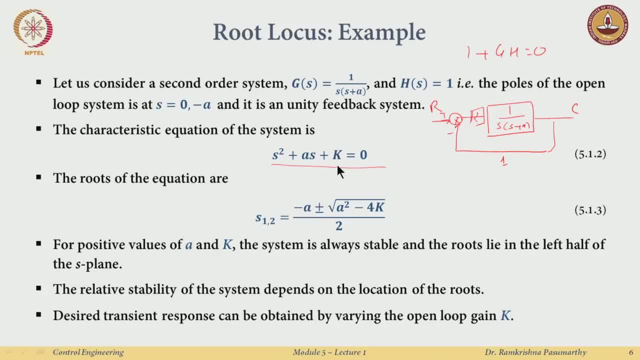 for given zeta and omega n, which was always positive. we never worried about stability because stability was very obvious in that case. right, You can now see that the route criterion satisfies this very trivially and therefore we were really never worried about stability. ok, 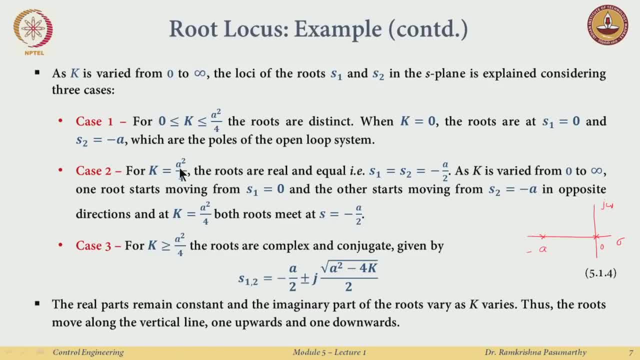 For k equal to a square by 4, this guy disappears and I have equal roots: minus a by 2, minus a at, minus a by 2. ok, So let me just say that these are when k equal to 0, k equal. 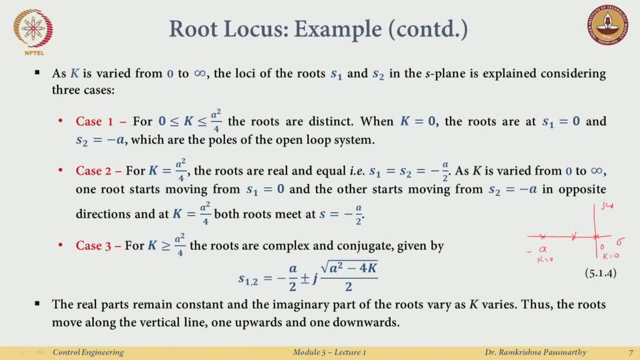 to 0, and when k equal to a square by 4, well, this is at minus. a over 2 occurs at k equal to 0. So when k changes from 0 till at least it reaches a square by 4, what I see that this? 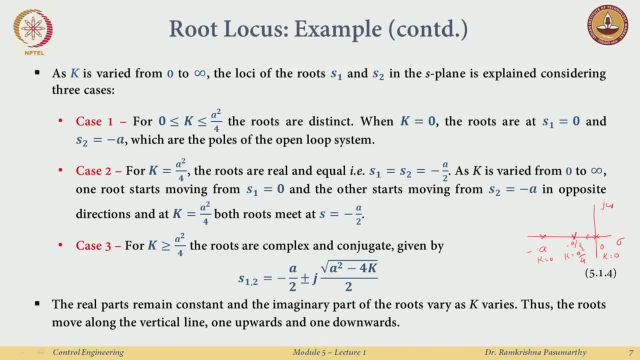 guy starts moving here and this guy starts moving here until they both meet at this point, right at a square, at k equal to a square over 2, and this point, which is minus a over 2, ok, Ok, Now what happens after this? it is ok- was between 0 and a square by 4, well, I just say. 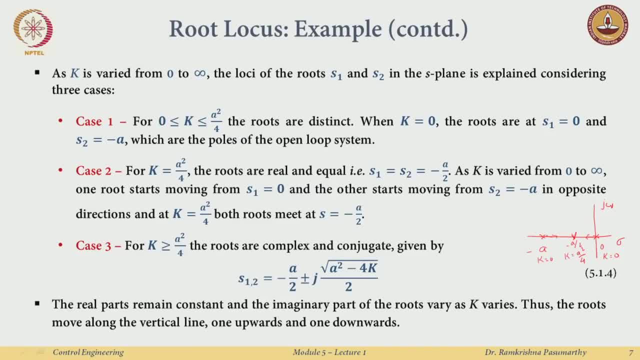 that these are somewhere here. Well, I knew that they were somewhere on the real line, but now I know that even k equal to a 4 know they meet here. So this guy travels here. this guy travels here. what happens for k being greater than a by 4?? Well, the roots. 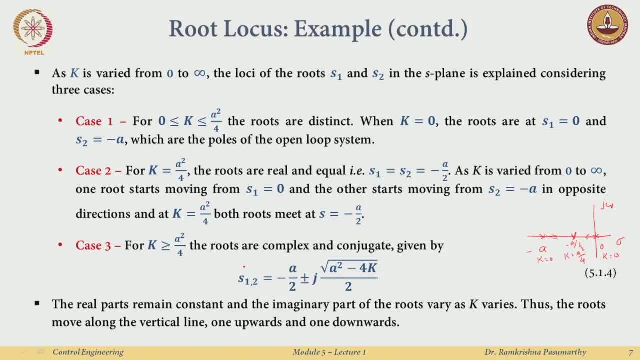 are complex and conjugate and given by this number. So what you see? that after k becomes greater than a by 4, a is given to us right. So this guy remains fixed. ok, So all the real parts will be at minus a by 2 and the complex part. 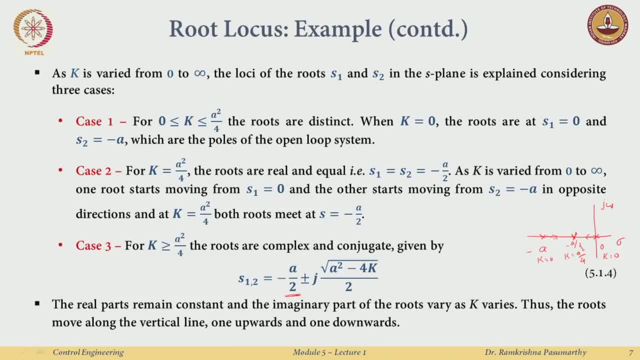 will follow this guy, which means, well, I am just So there will be. all the real parts are a by 2 here and the complex parts will keep on changing. So when k equal to a k equal to a square by 4, I am here, and then I see that I am just moving around this lines. 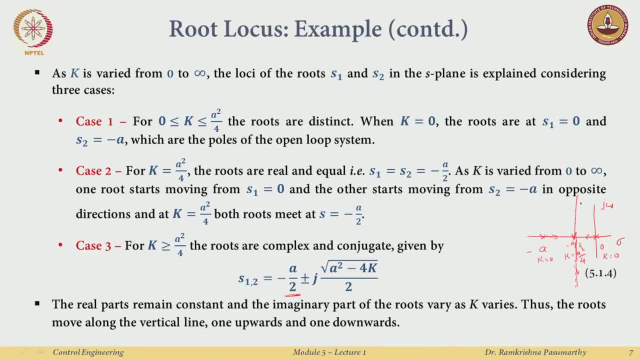 this lines and this lines. ok, So this is for k greater than a square by 4. similarly here, k greater than a square by 4, and we know that if there is a root here, there will always be a root here, right? because of the nature of the system, right? 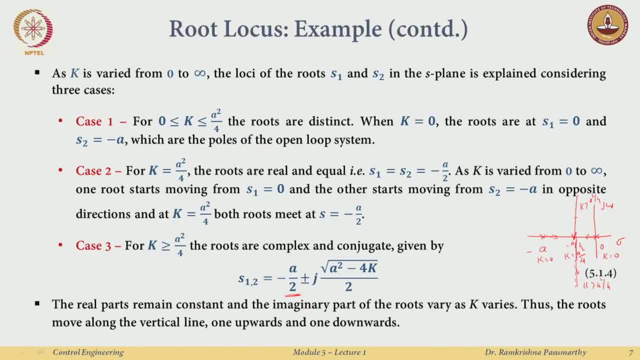 So the real part remains constant and the imaginary part varies at the gain k varies. Thus, the roots move along a vertical line, right here, 1, 1.. So they go this way and this way. So what do we observe right? So, as gain k for k equal to 0- I am just at the open. 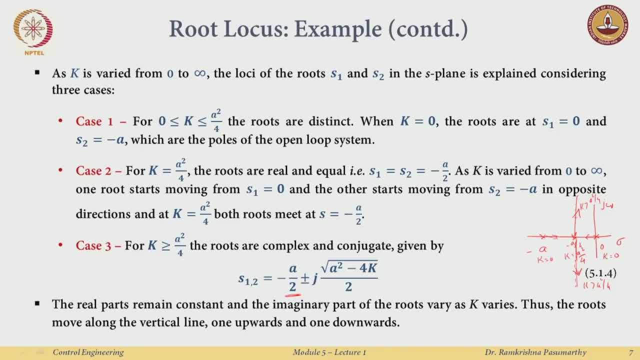 loop poles. ok, As k increases, both these guys meet up here and they again go away right to. they will just keep going till infinity. ok, So something nice happen is happening here, right? So what information I used? I just used this guy g is s sorry, this is 1 over s s plus a right. I am not doing anything. 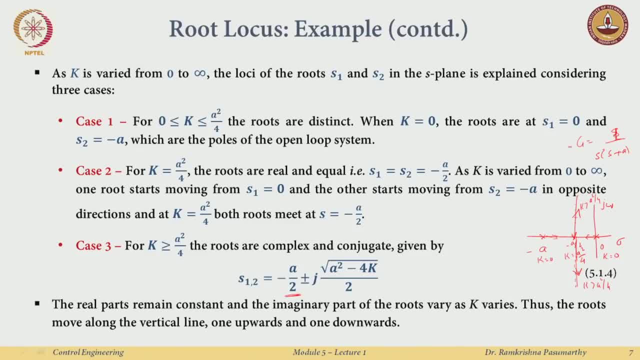 with the transfer, with the characteristic equation now, and I am just interested in how this k times g, and then now this will be the closed loop. ok, I am not draw this out, So I am just taking this information right. this is this guy. ok, 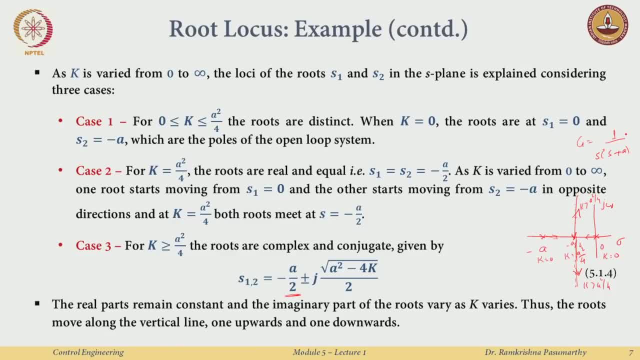 Ok, Thank you, Thank you, Thank you. So what I observe for k equal to 0, I am at the open loop poles and as k increases, these guys tend to move and they direct, they decide to move, they decide to meet here and then. 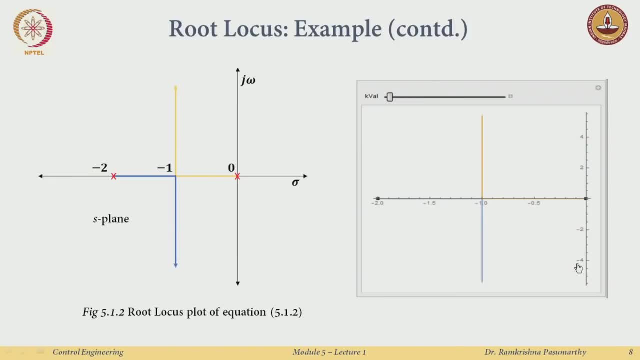 again separate. ok, So this is how. if I just play a very small video of this, right? So this is how the roots will go. something is ok, right? So if I give so again, I will just play this again, Right? 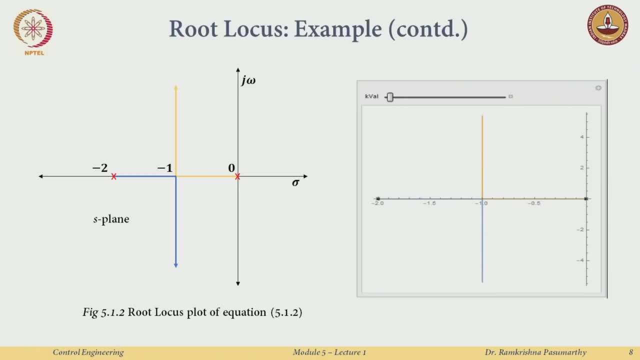 So this guy will go and then for log values of k and then go small and then again come back to the position. ok, So this is how the roots will move. So this guy will go here and move this guy direction. this guy will go here and move this direction. right, ok? 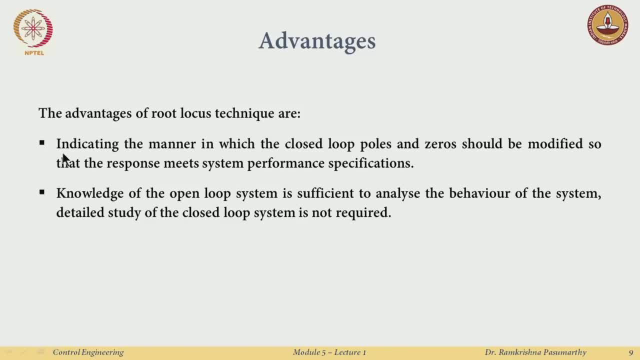 So what did we know? what did we see here? that So the root locus. it indicates the manner in which the closed loop zeros and poles move, So that the response meets some specifications. So my specifications are usually in terms of zeta and omega n and these specifications. 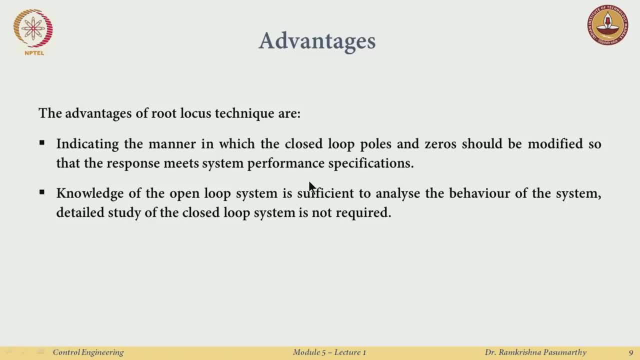 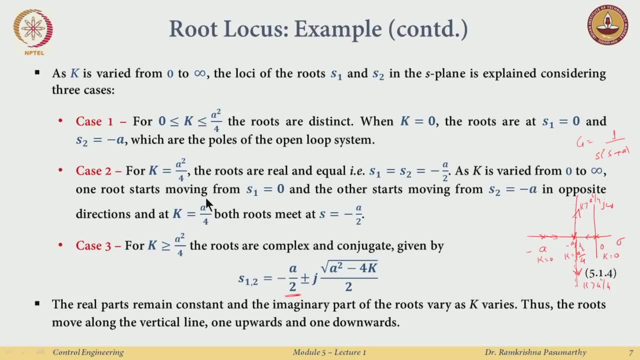 usually translate to locations of poles. So this could be some zeta and omega n, which would be: may be satisfied by k equal to a square by 4 plus 1. right, then I would know. right, So I will exactly know where the roots are. may be somewhere here and somewhere here. 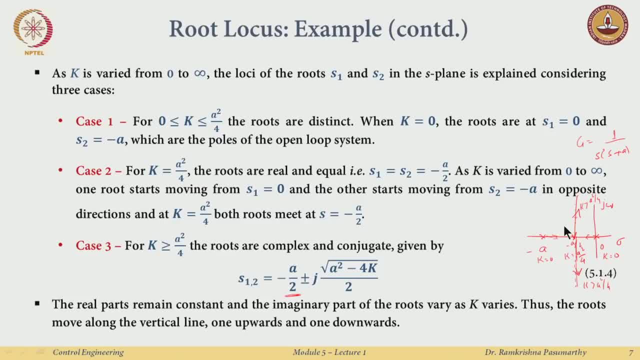 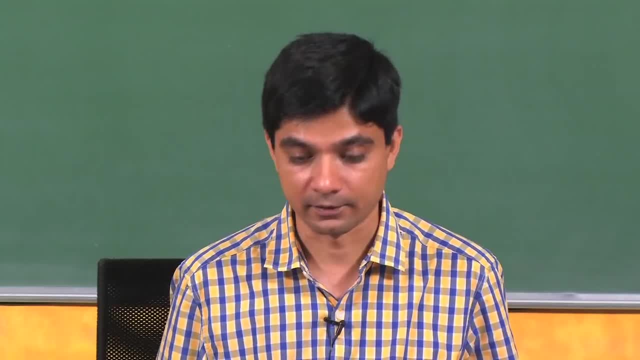 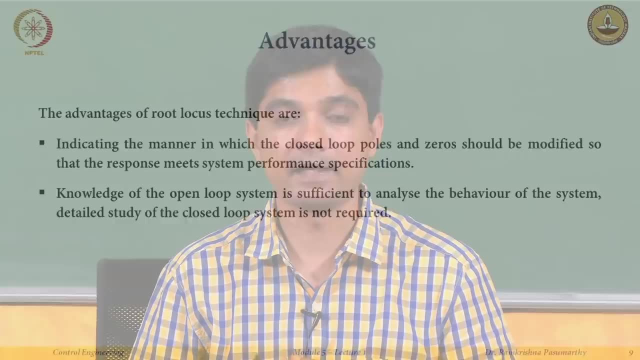 right, and then I would actually exactly know what should be the value of k, such that my closed loop poles satisfy some. So some desired specifications or some desired performance criteria, ok, So I would know how to modify the gain k such that my performance is met and performance is usually mapped to. 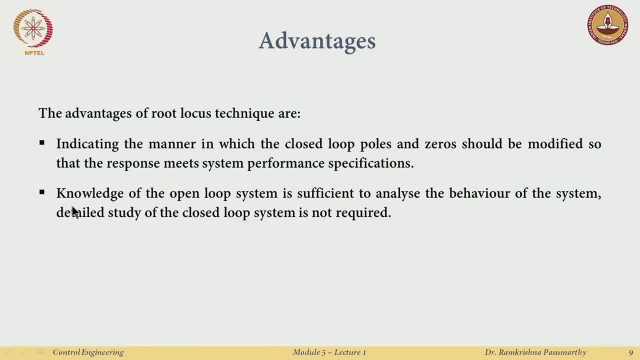 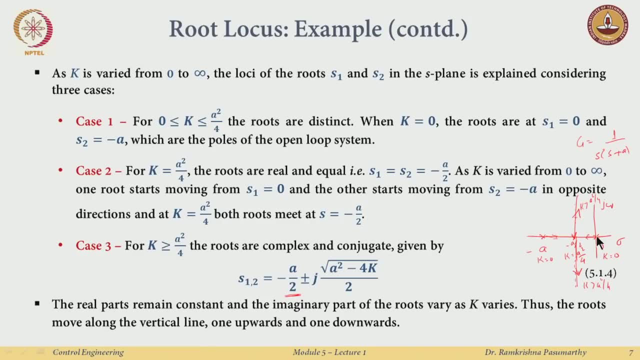 some pole locations. ok, And I am just doing this only with the knowledge of this guy, right, I started with s, the open loop poles, s at 0, s at minus a, and I am just Increasing the gain k. we will see how we will formalize this a little later. So just, 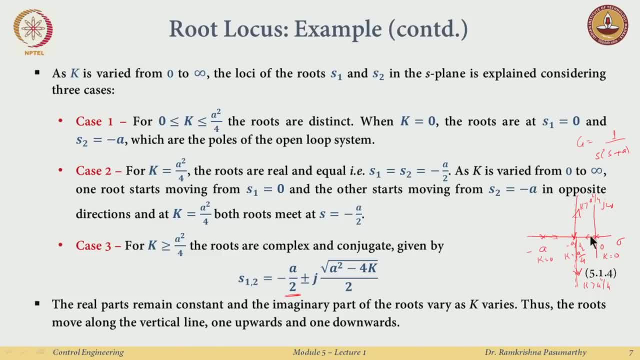 by looking at these two. I start with the open loop poles and these are all the closed loop things now, right, as k increases- I am already in the closed loop right- and then how the closed loop poles are modified, starting from the open loop poles. So I just need to know: 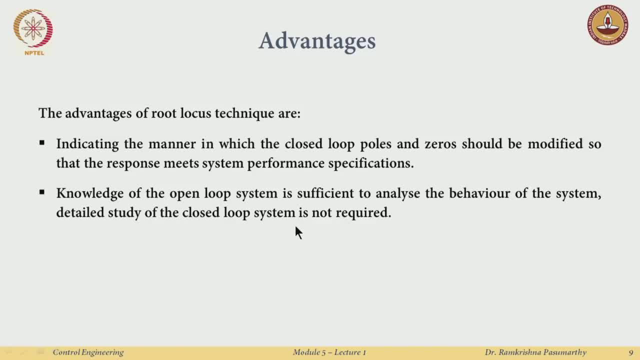 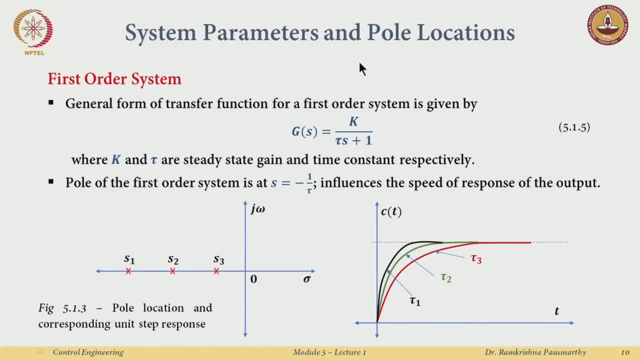 how the open loop system looks like and I can just do a good study of the closed loop system So I can compute the closed loop poles and then I analyze things and so on. right, So how are poles related to pole locations, related to the, to the performance? well, we analyzed. 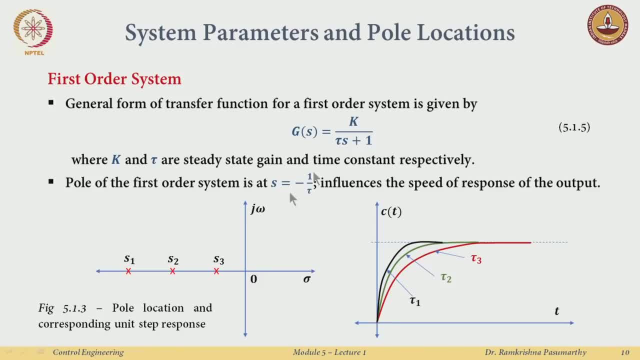 this while we were doing first order systems. So just say, if for different values of poles, at s 1 I will have faster response, s 2 slightly slower, and the slowest will be for s 3, right? So how? the, how the location of poles influence the performance? this we did while we were 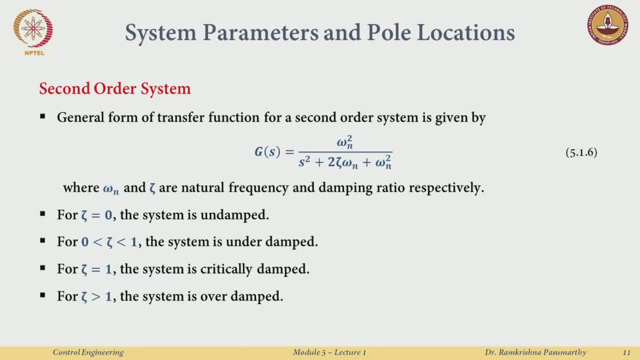 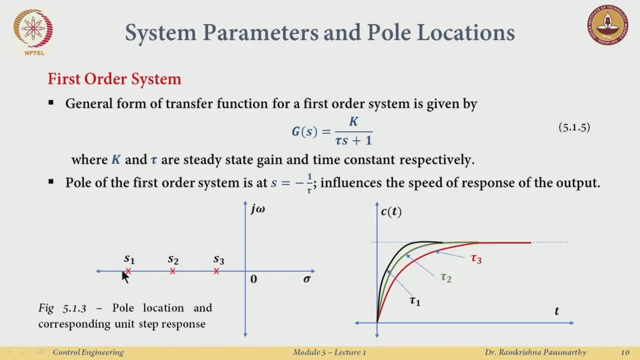 doing analysis of first order systems. ok, Now in general. so the first order system was very easy, right? So all the poles are on the real line. then, based on their location, I would determine how are they fast? are they slow? the slowest would be here and the fastest 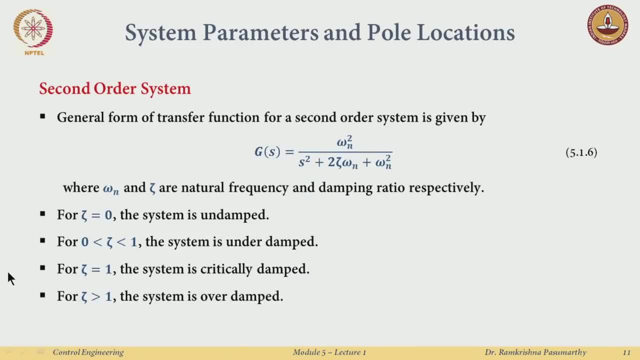 would be very, you know, further away from the origin. ok, However, for second order systems, there were little, Little, Little more details. right, We started. well, we had this un-damped systems, where we had the maximum overshoot. the settling time was infinity. then we had the case of underdamped. 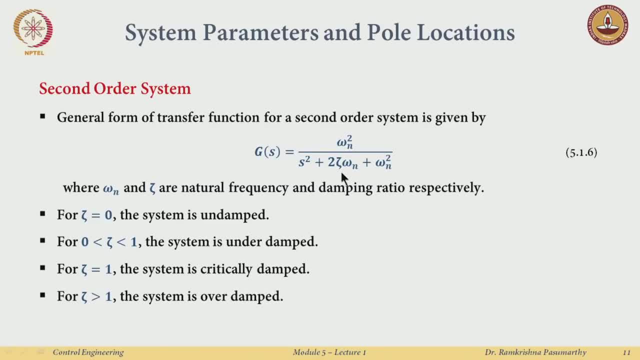 systems where we quantified, you know, where we define underdamped nature in terms of zeta right. and then we had also, when the system was un-damped, the, the frequency of oscillation was omega n, for sigma equal to 1, the system was critically damped. and then we also had 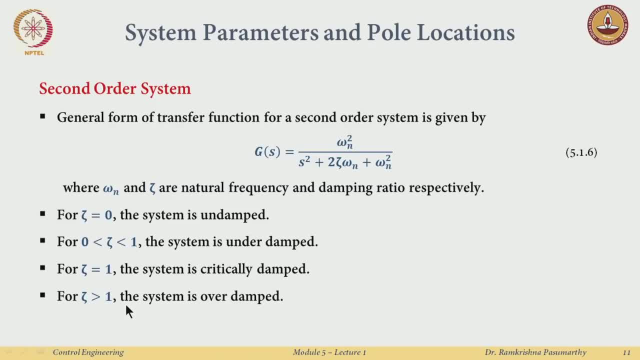 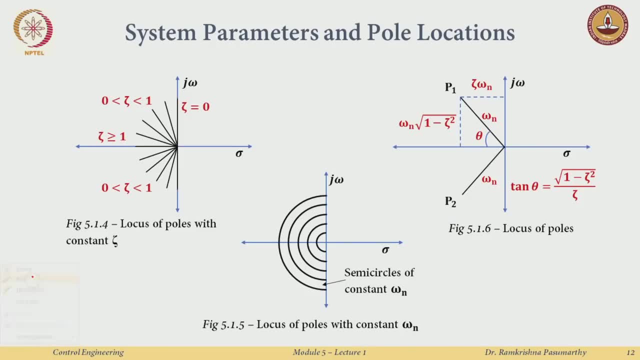 the notion of of over damped system, where this, So it was greater than 1. ok, So if I just look at, you know the poles, I typically. well, I am just looking at solution to this equation at s square plus 2, zeta omega n, s plus omega. 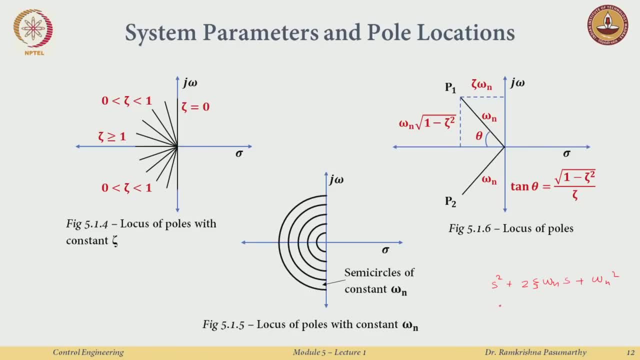 n square. ok, So if I just look at the underdamped case, my roots were minus zeta omega n plus minus j omega n square root 1 minus zeta square. So this is for zeta less than 1, if I, if I. 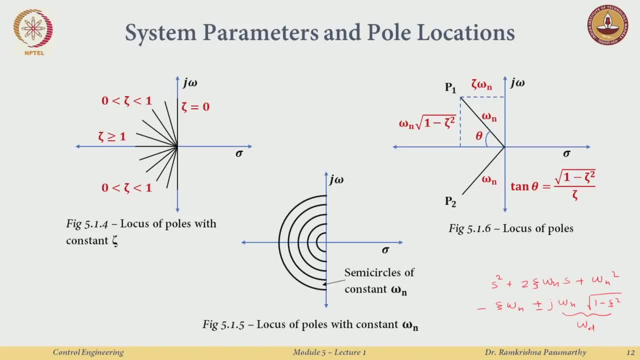 remember it properly, and this guy I said: this is omega d. ok, So this is the real part here. So if I just take a complex, a conjugate pair at p 1 and p 2, the real part this distance would be: this will be at minus zeta omega n and this is. 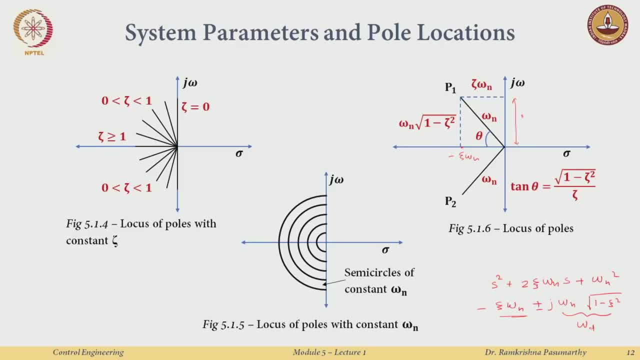 then this guy would be omega d, this distance, Omega d is omega n, square root, 1, minus zeta square right. this is just like. So this is a right angle triangle and I could say that this omega n is just, you know, square root of this guy, plus this guy right from the Pythagoras. 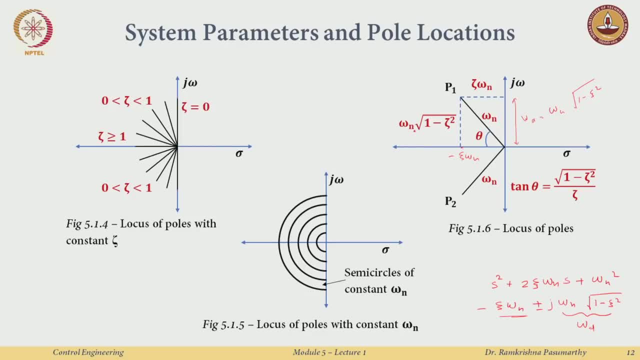 theorem. ok, Now something else, right. So this is what we also called as the omega d, right. ok, Now look at this guy, theta, right. and if I say, how does cos of theta look? like Cos of theta, is this guy zeta? omega n over omega n is just. 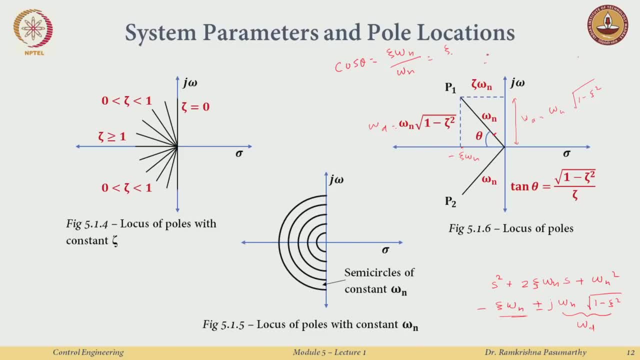 zeta, right? ok? So from this, cos of theta is zeta and therefore theta is cos inverse of zeta, right? So from this, cos of theta is zeta and therefore theta is cos inverse of zeta. ok, So let us look at this right? So if I am at this point, theta remains the. 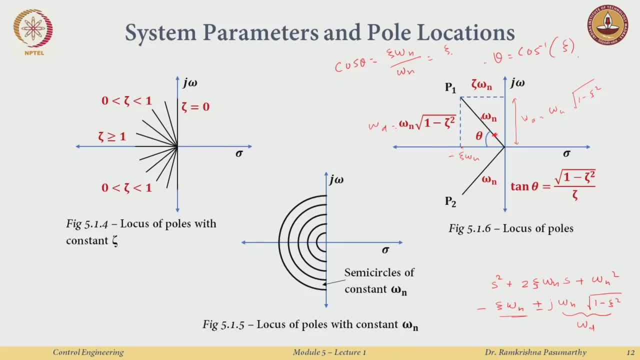 same, whereas omega n changes. right, If I go here. if theta is the same, then zeta is the same. ok, Now, if I go from here till here, this distance, which is omega n, changes, but cos of theta still remains the same. right, slightly here also, if I go from here till. 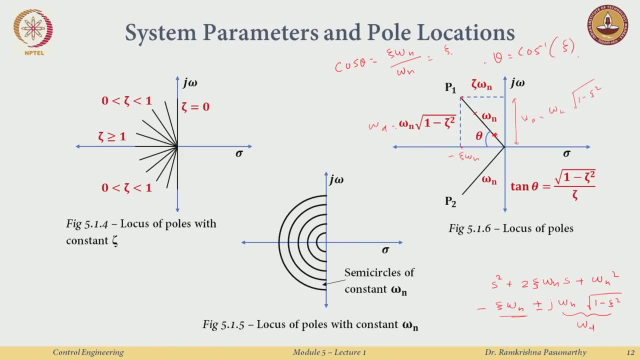 here what happens? So my zeta remains the same because theta is the same, right, if I am just moving along this line right and then omega n changes, right first for some given zeta. So all these lines are lines which I call as constant zeta lines. So I can go here if I just take any arbitrary 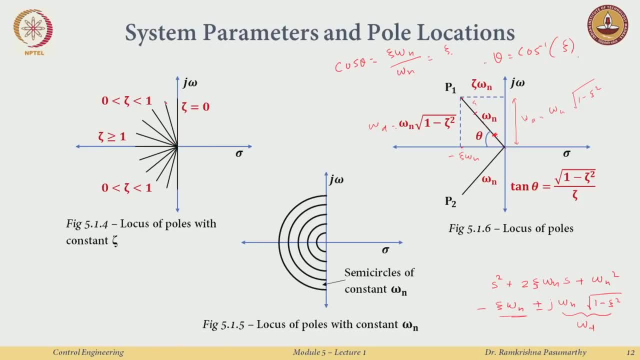 line here right, for which a theta would be fixed. If I move along this line, right, what happens단 my theta is fixed whereas omega n changes. ok, So this behavior could be seen from zeta equal to 0, I am here, I keep on increasing zeta, and there are all these lines. are the? 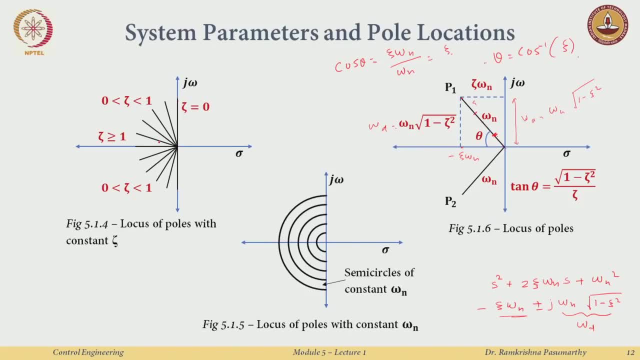 lines for which the zeta remains constant. So at this point you will have different omega n, this point, different omega n, but the zeta here is same, similarly on the other side. ok, So these are all constant zeta lines, or we? 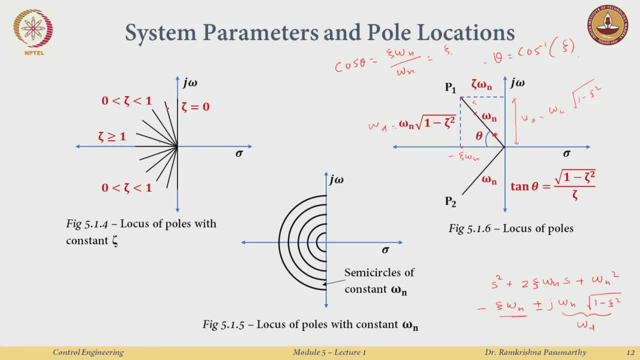 just say how the locus of the poles look like for constant zeta. ok, Now let me keep omega n fixed and keep moving right, and I just want to vary theta. So what will I do where omega n is fixed? omega n is fixed and I just move around some semicircles. I do not want to. 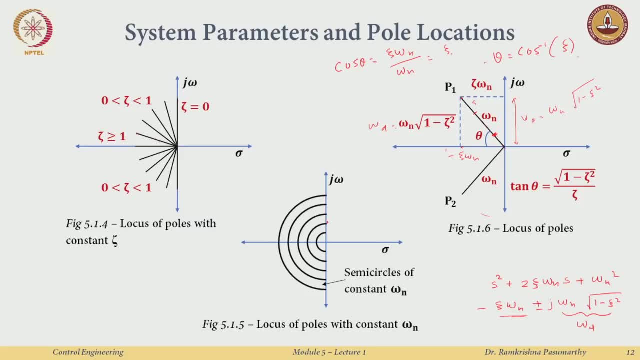 do a circle because I do not want to go into the unstable region. So if you look at this guy over here, omega n is same, omega n is same, omega n is same, same, but each of this will have different zeta right. 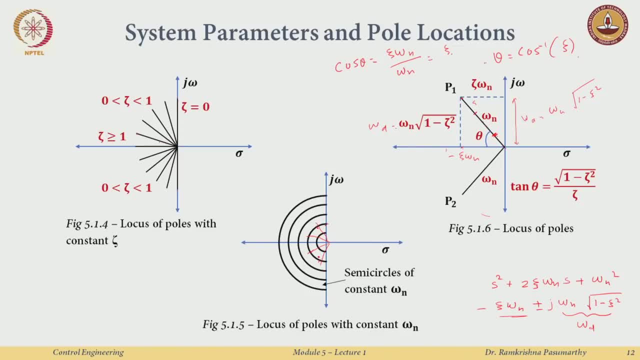 This will have a different angle. this will have a different angle and this will have a different angle. So if I, if I keep on moving omega n, then I just see, I just move, move, I am just moving around the circle, and this guy also, you know, since all poles exist in. 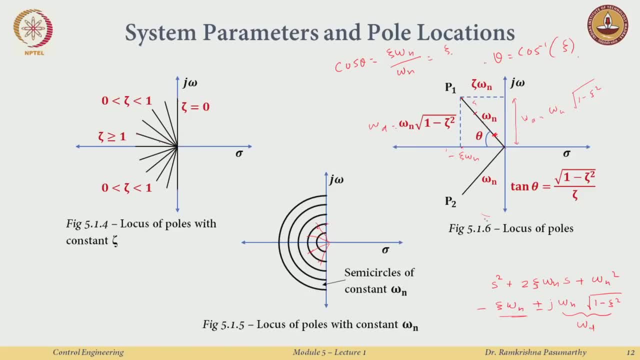 complex conjugate pairs. So this guy will also move, moves just according to how the omega n varies. So you just have some semicircles here. So there is a pole here. there is also a pole here and this will correspond to certain zeta. 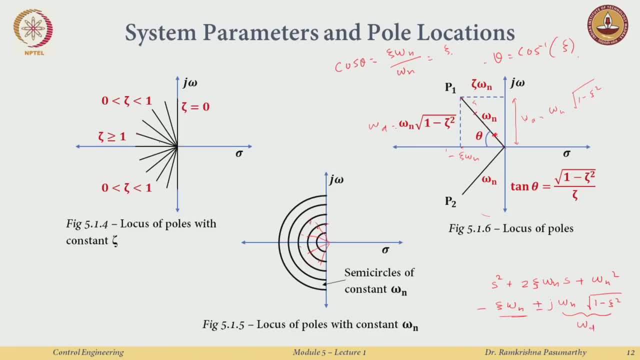 If I go here, This pole will move here and this pole will keep on. will move here right the complex conjugate, but in the zeta will move. So these are semicircles of where omega n is constant and zeta is changing. 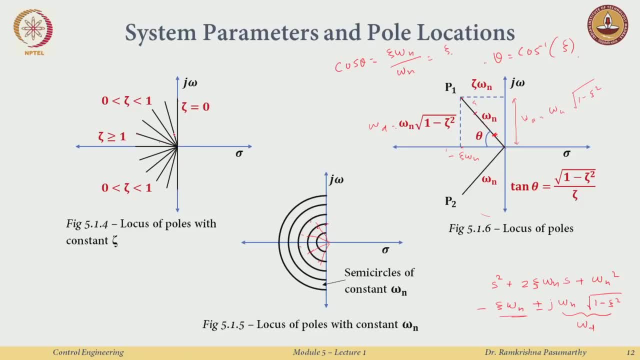 These are lines where zeta is constant and omega n is changing. right, ok, What is? what is the importance of this? When I say we will design something such that zeta is some number, And And, And, And the omega and the omega n is also some number. say, zeta is a 45 degrees and omega 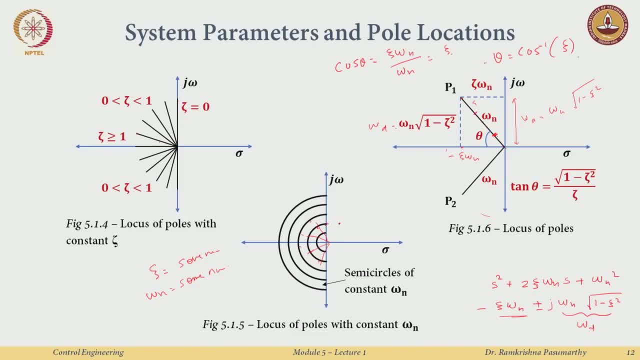 n is 1. ok, So I have this constant omega n circles and then I just draw a line of say zeta, or say the theta being 45 degrees. So just draw a line from here till here and if say this is omega n equal to 1, then my pole should be here. ok, So if I have like I will. 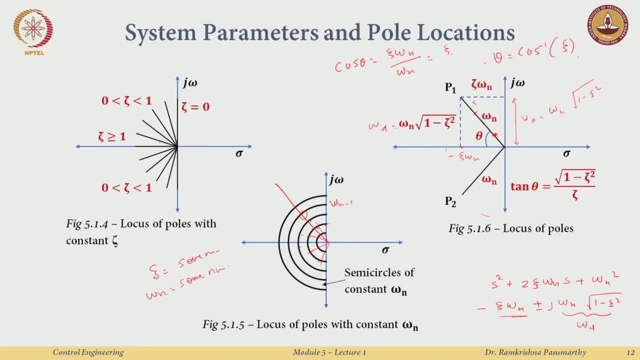 repeat, want a design specification where zeta should be, say some number which corresponds to angle of 45 degrees. given a given theta, I can always compute zeta right and then, and a certain omega. let us say this is 1. So I just find these 2 lines. So this is my zeta right and 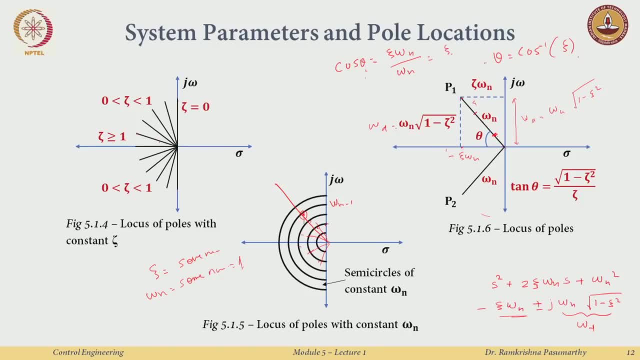 then this is my omega n equal to 1, and the point where the intersect is where I want my closed loop poles to lie, and this I know how. you know from the previous example that I could vary these closed loop poles just by, you know, varying the gain. 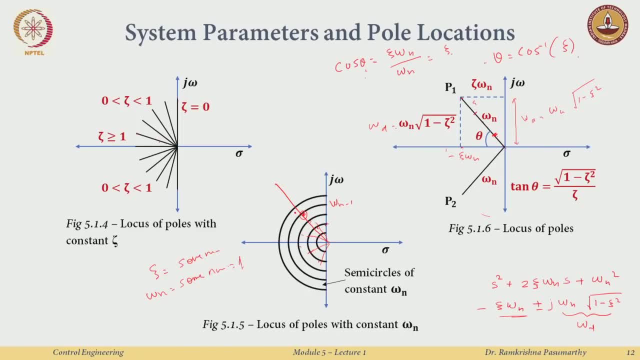 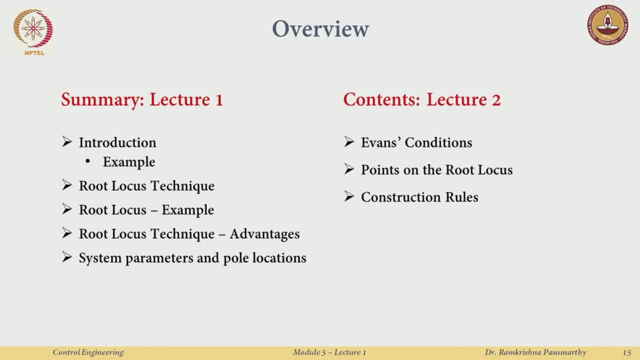 Now I will just investigate. is there any gain which will do with me this? Now, how do I test? right? So that is exactly what we will study in the root locus case. ok, So this was just a little example, right, and now we will see how we can generalize this, right. 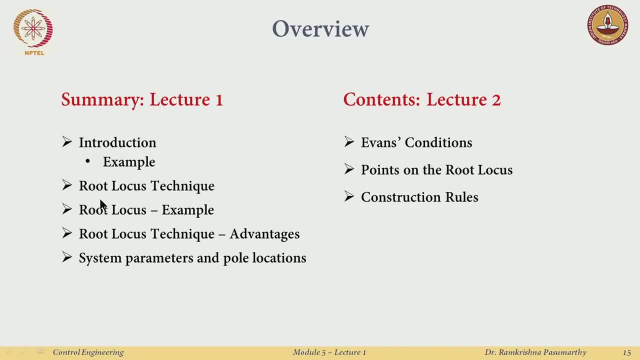 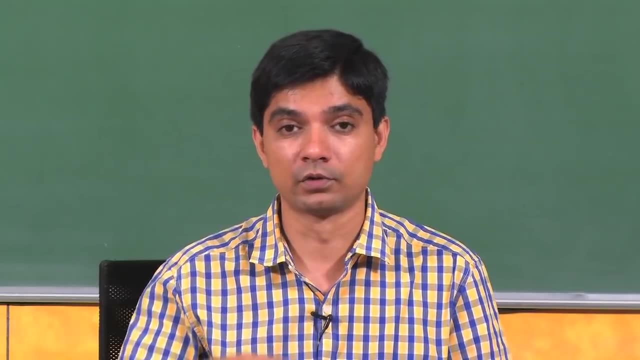 do the roots. So what we saw? that the roots were travelling towards each other. they meet and then they go away. do they always meet? and if they meet, do they again have to go? do, do. Do they have to go to the imaginary axis, or they could possibly just stay over there?